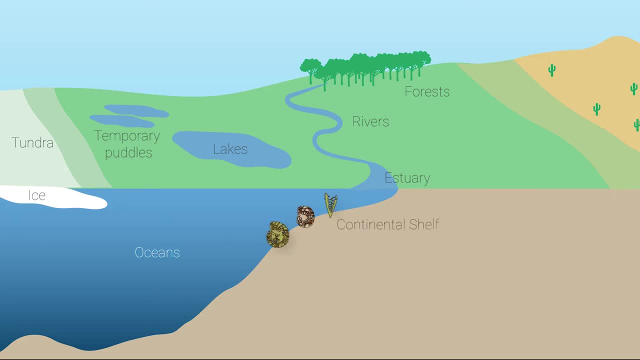 In addition, different species of Benthic Foraminifera live on the continental shelf, the continental slope and on the abyssal plain. Knowing which species occur at which water depths in the modern sediments allows paleontologists to use the remains of Foraminifera to determine. 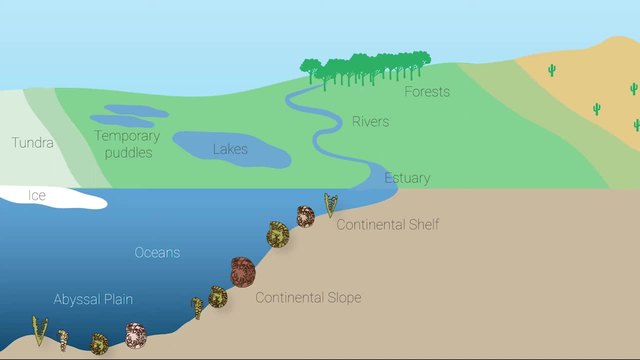 past changes in sea level along coasts. With this data, they can predict how sea levels will change in the future. Different types of Foraminifera also respond to changes in food and oxygen availability. Foraminifera live on the seafloor. By examining the changes in Foraminifera in ancient sediments. 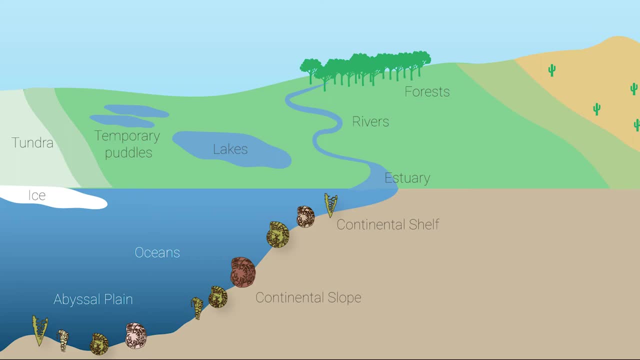 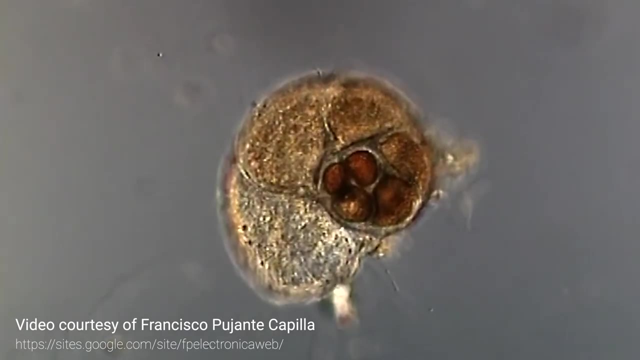 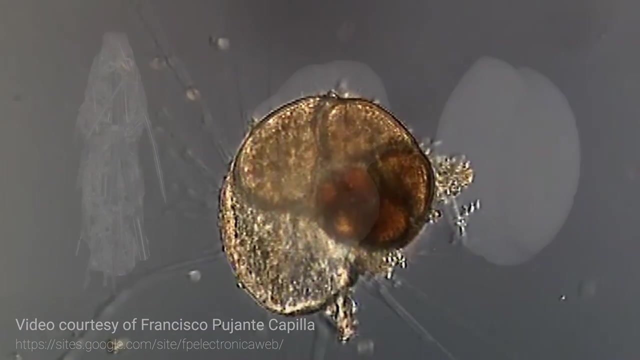 we can reconstruct how oxygen and food availability changed with ancient climate changes and understand how modern climate change will affect ocean ecosystems. This video will focus on the morphological characteristics of Benthic Foraminifera that micropaleontologists use to differentiate among different species and reconstruct ancient environments. 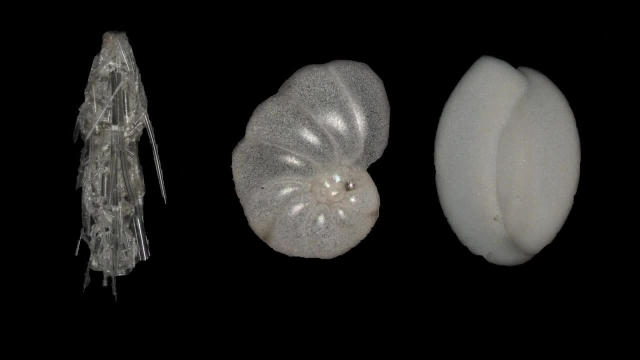 Among Benthic Foraminifera. the first characteristic important for identifying major species groups is the material from which the Foraminifera live. The first characteristic important for identifying major species groups is the material from which the Foraminifera live. 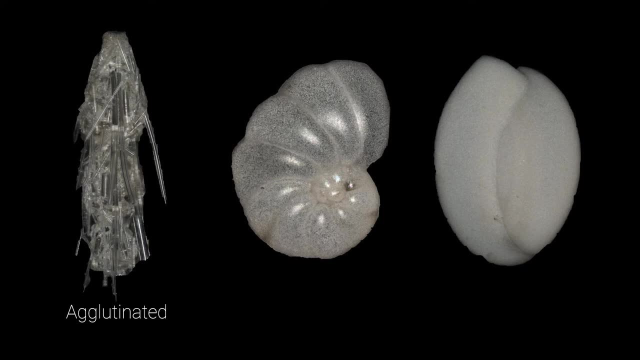 Agglutinated Foraminifera embed sediment, grains and the remains of other organisms into an organic matrix to make their shells. Both Hyaline and Porcellanus Foraminifera use carbonate to make their shells, but Porcellanus Foraminifera have a smooth, opaque shell, whereas Hyaline. 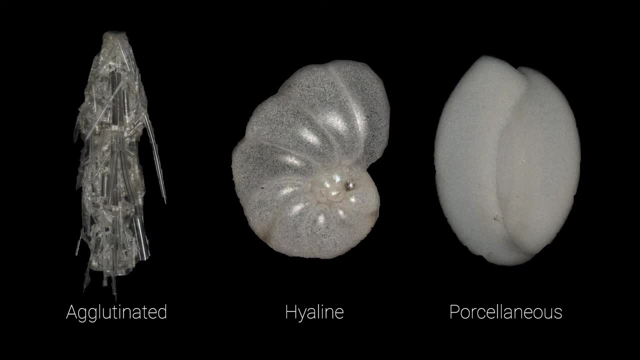 Foraminifera are dotted with pores and often translucent. Just identifying these different shell types can help reconstruct the salinity of ancient bays and estuaries. Porcellanus Foraminifera are most abundant in hypersaline environments, while agglutinated Foraminifera dominate brackish. 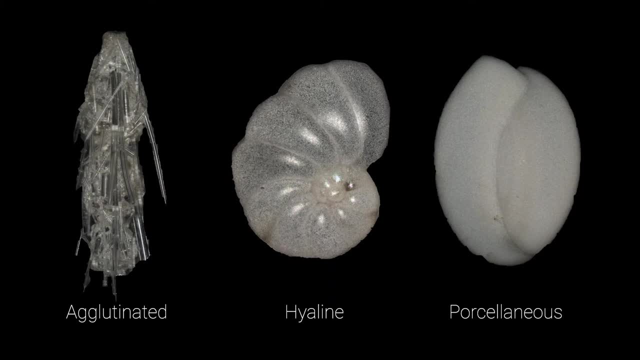 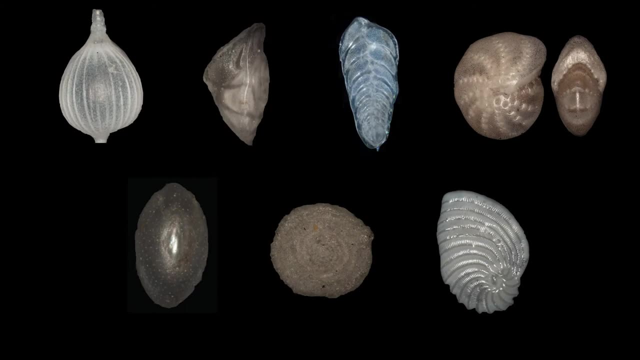 water environments and Hyaline Foraminifera are most common in normal marine conditions. The shapes of the overall Foraminifera are very diverse and is the second thing you should observe when trying to identify a species. Foraminifera may have a shape like a vase or a cone. 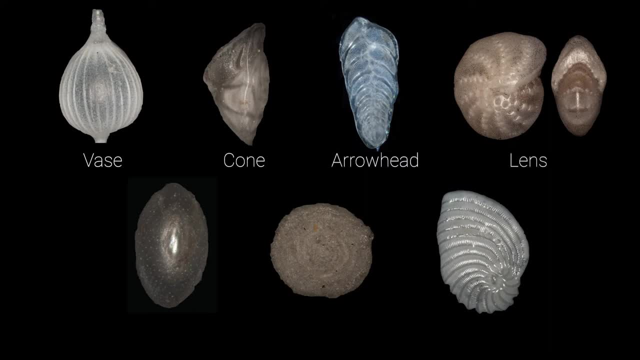 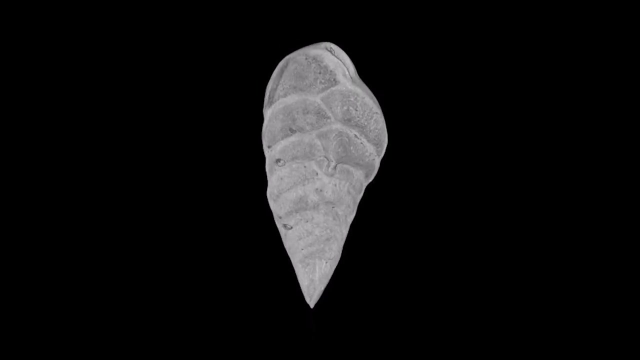 or an arrowhead or a lens, an oval, a disc or a fan, among many other potential shapes. As you examine the overall shape, you may need to look at the Foraminifera from a few angles to understand its shape in three dimensions. 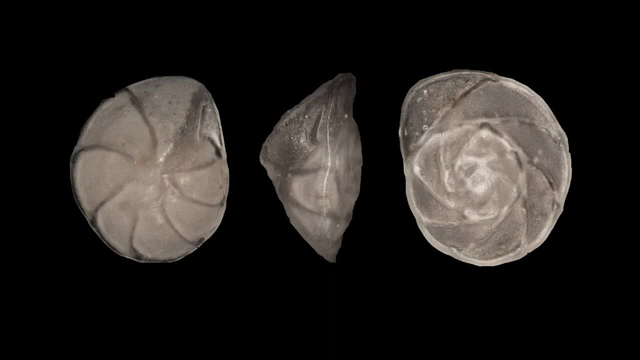 To help you visualize the Foraminifera in three dimensions, the images you will see will show three views of each specimen In the form shown here. you see its umbilical side, an edge view with the aperture facing outward, its spiral side and its spiral side. 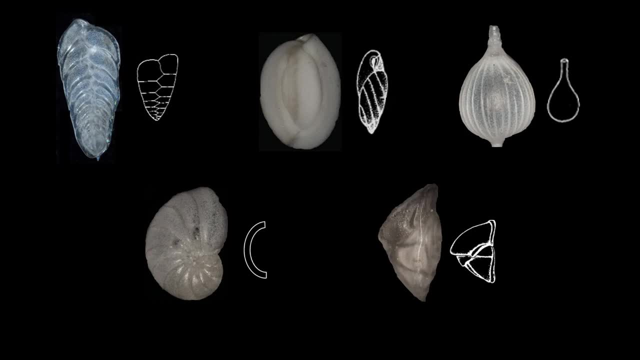 Most Foraminifera grow by adding chambers to their shell to accommodate the growing cellular material that makes up the organism itself. Sometimes the chambers are shaped like short and broad boxes and other times they are long and thin, with the long axis of the chamber. 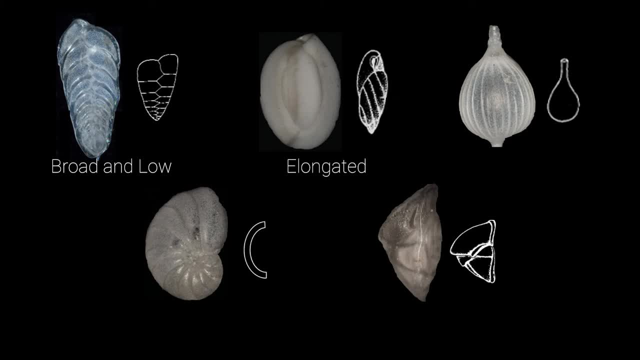 parallel with the long axis of the overall Foraminifera. The chambers may also be inflated and globose, with rounded chamber walls shaped like arches, or have walls that meet at sharp angles. In this example, the Foraminifera is shaped like a circle, but it is also shaped like an arch. Some 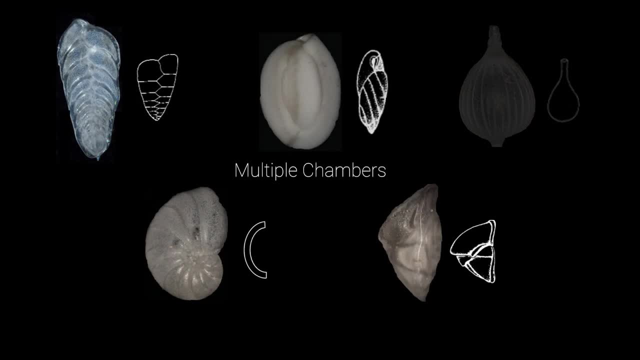 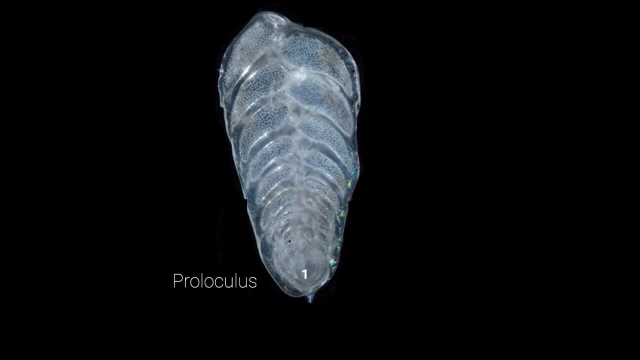 Some foraminifera have only one chamber, while others may have dozens of visible chambers. The first initial chamber, or proloculus, of a foraminifera is nearly spherical in shape and chambers are added as the foraminifera grows. 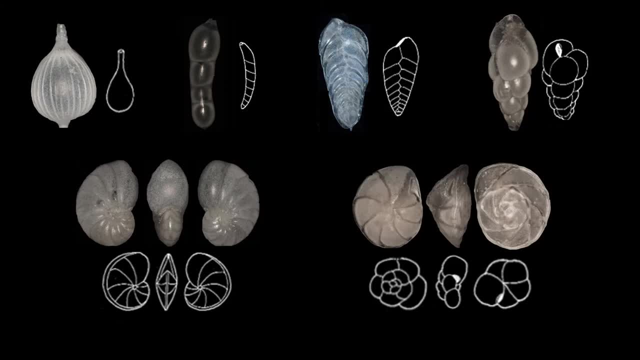 The pattern by which chambers are added determines the overall shape of foraminiferal shell and varies across genera. This is one of the most important morphological characteristics to recognize when trying to identify a foraminifera. Unilocular foraminifera have only one chamber. Others add chambers in a single row or column and are called uniserial. 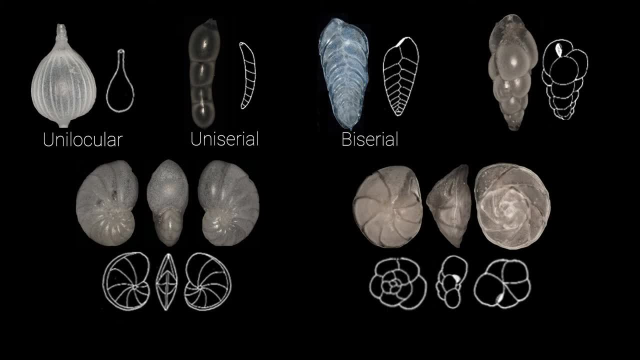 Biserial foraminifera have two rows of chambers added on either side of a central axis. Tricerial foraminifera have three rows of chambers which sometimes appear to twist around each other. as the chambers get larger over time, Some foraminifera coil in two dimensions, creating an expanding spiral outward from the initial chamber. 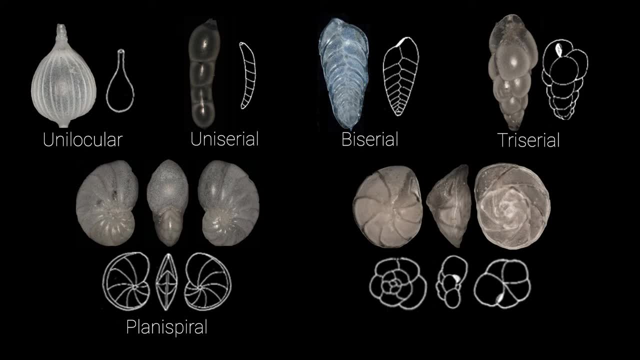 If the coiling is offset in a third dimension, coiling outward and upward at the same time, this creates a cone shape and is called a trochospiral chamber arrangement. Some foraminifera even combine these arrangements, transitioning from tricerial to biserial over the lifespan of an individual, or adding chambers along two rows, like a biserial, while also coiling. 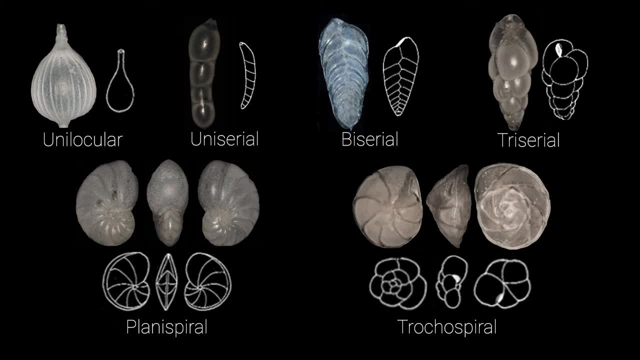 These different morphologies reflect the different lifestyles of the foraminifera related to the environments in which they live. For example, biserial and tricerial foraminifera often live deeper within the sediment than other forms and are more tolerant of low oxygen conditions.